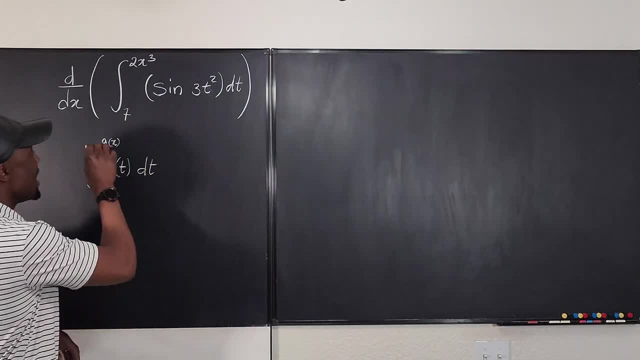 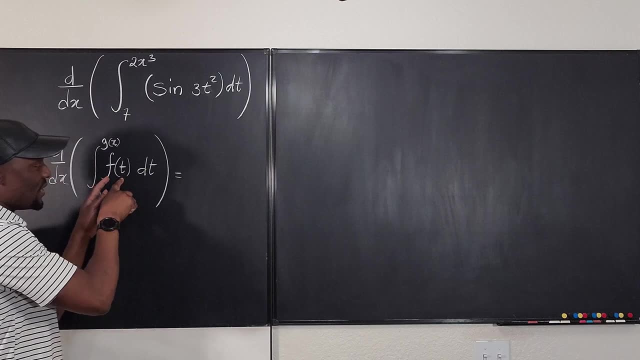 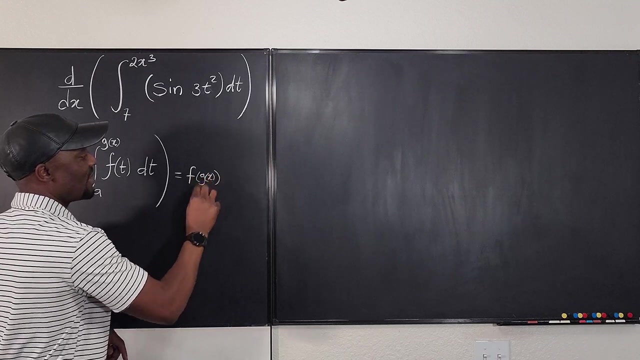 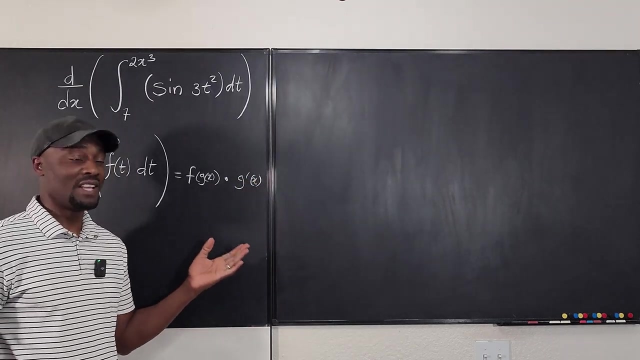 function of x. once you have this expression, if you take the derivative of this, all you're gonna get will be this function, but now in terms of g of x. okay, multiplied by the derivative of g of x. this is the part that many students do not realize. 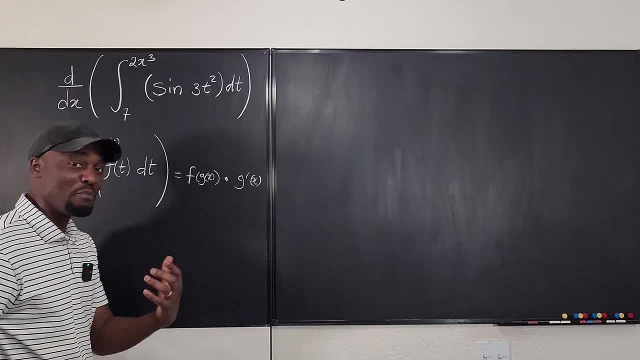 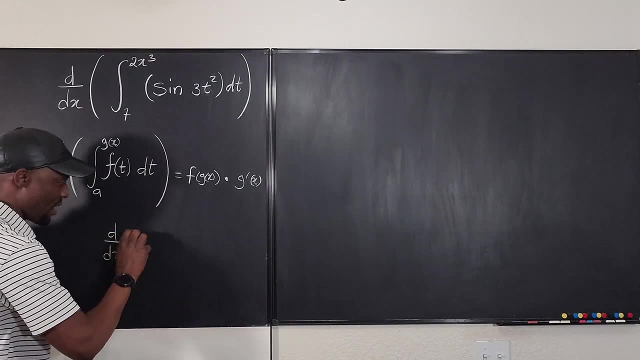 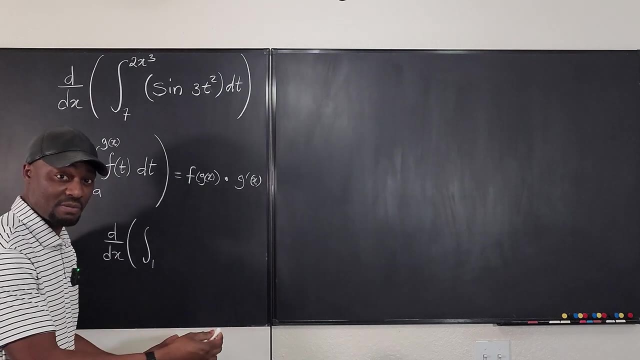 that when you differentiate this, this is what you get, because what most students see is they just see x. let me explain to you. so let's say this expression was d, dx of the integral from say one. so this doesn't matter as long as it's a constant. it's not a variable from one to x of. let's say: 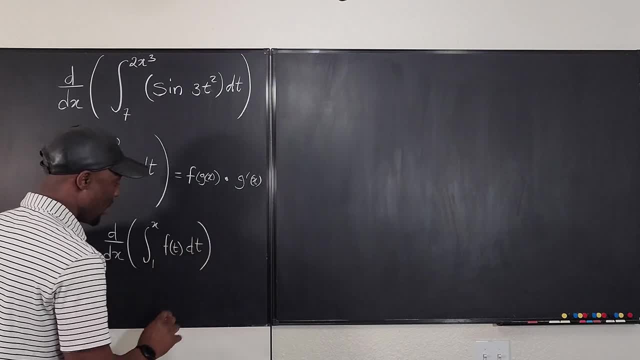 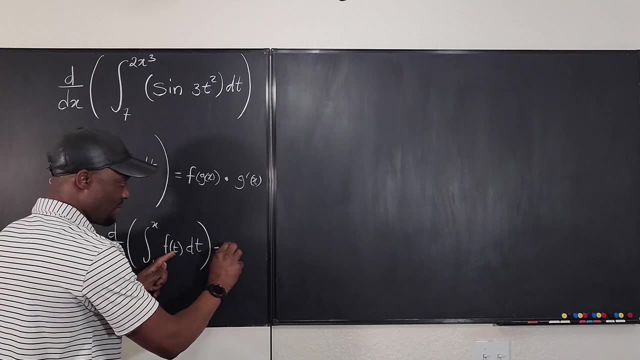 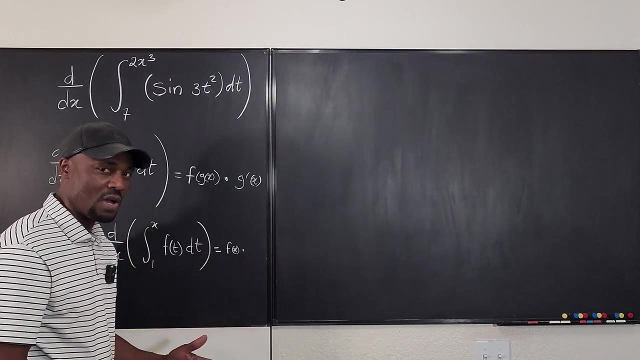 f of t, dt. what you have here usually turns out to be this same thing. this function replaces t, so it's going to be f of x, and then you multiply by the derivative of x, but the derivative of x is one, so most students stop here and think that all they 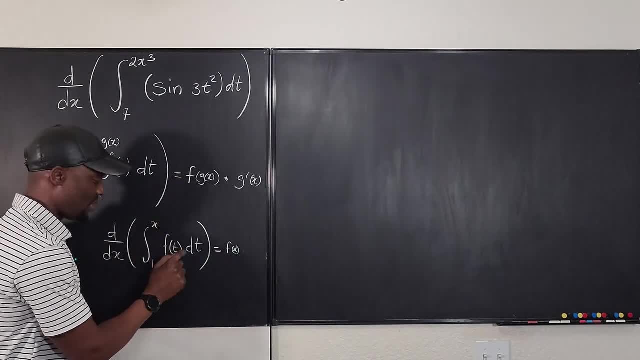 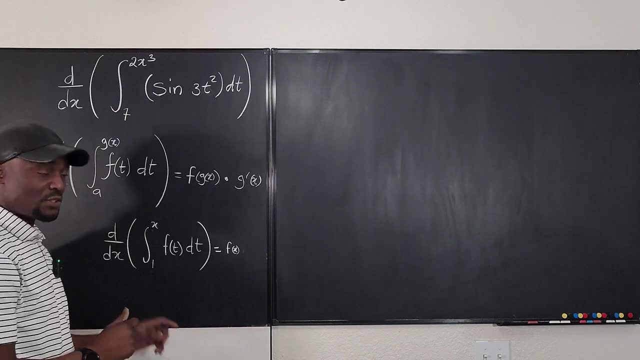 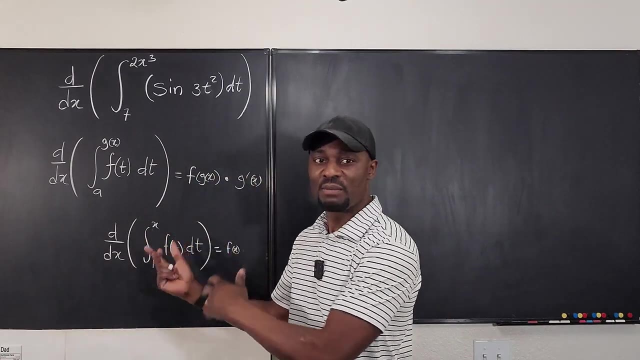 have to do is put this number- i mean this function here- and that's the answer. but no, you have to multiply by the derivative of the function sitting on top. so that is the fundamental theorem of calculus, part one. there's part two, which is actually which stems from part one, but part 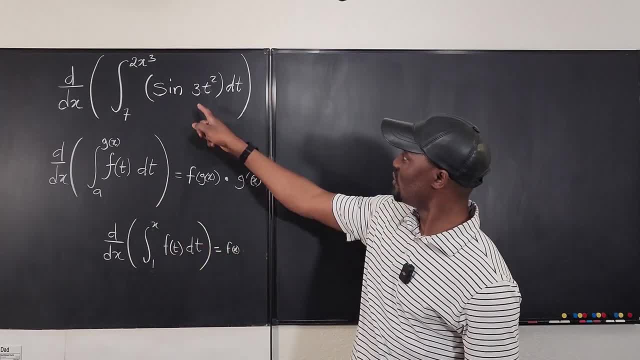 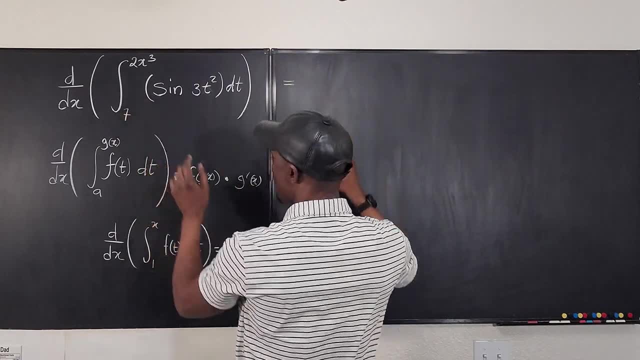 one is the part you want to focus on, and let's just use this to solve this. it's easy, straightforward. so here, what we have is this is going to be equal to we applied the same rule. we just have to, because this is a constant. okay, the number here is seven, so any. 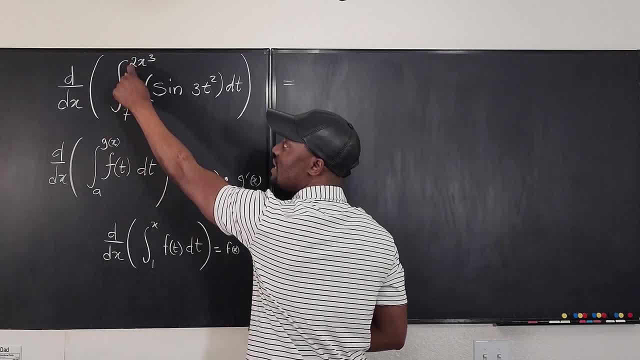 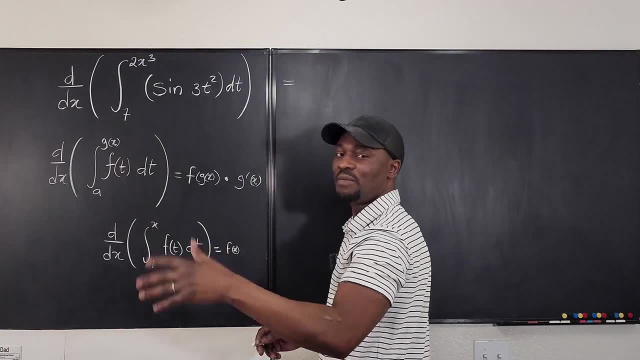 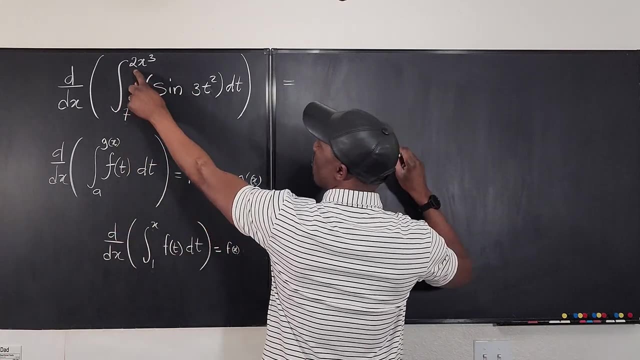 number could be here. you can't have a constant here. the constant has to be here. you have to have a function of x here and you have to have a constant here. okay, in other videos. i have another video that explains this. so this is going to be what we're going to replace t with. 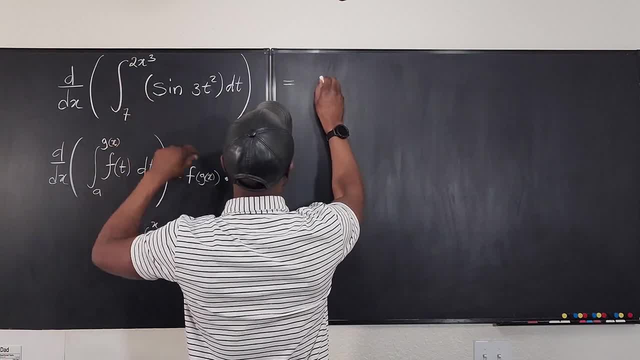 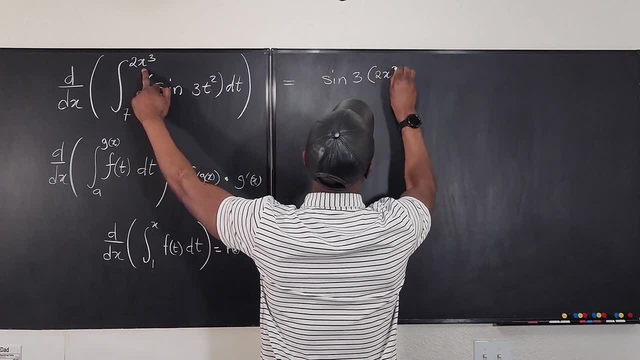 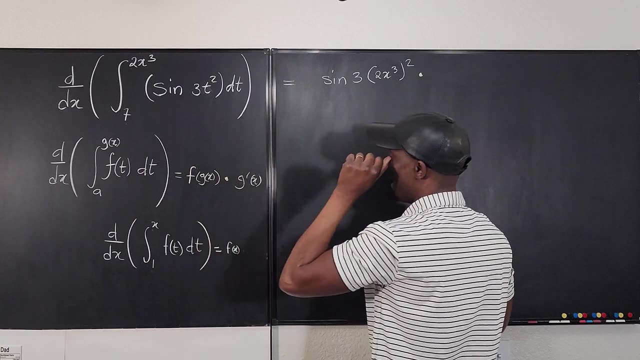 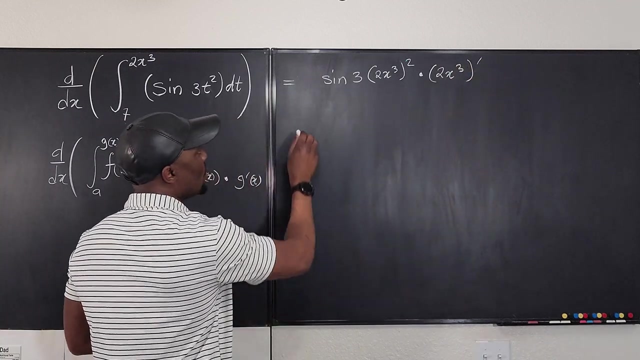 this entire function. so here we're going to have this to be sine three. the t will be replaced by two x cubed squared. you see that the t has been replaced, and then you have to multiply this by the derivative of this, which is the derivative of 2 x cubed this way. so what do we have? we have: